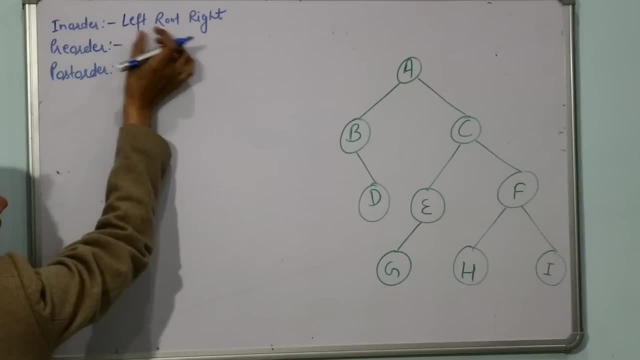 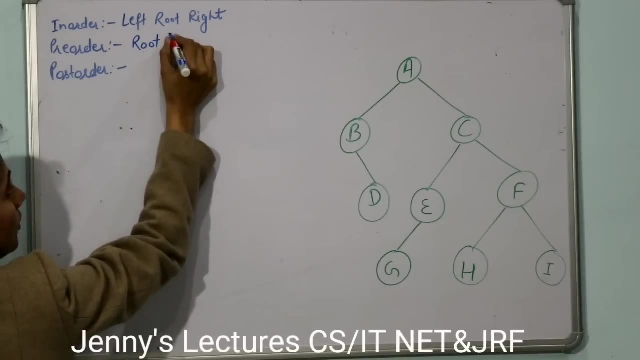 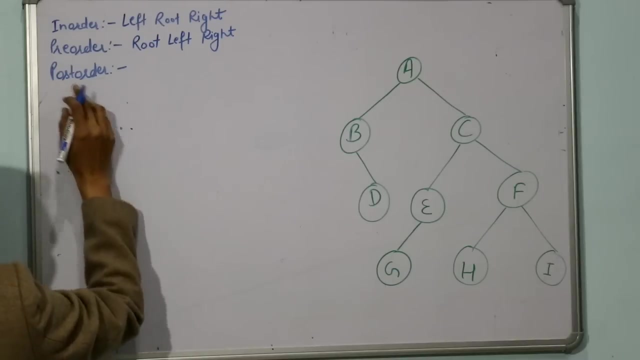 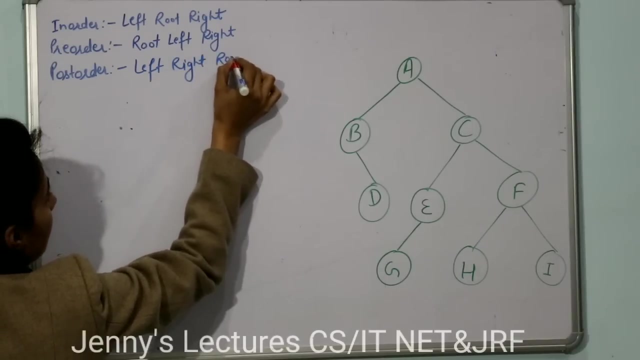 in or inside. you can say, then root would be in between left and right part. Pre pre means first. first is in that case what will happen here: traversal root, then left and then right. And what is post-order? post means later. So it would be left, right and root okay. In means: 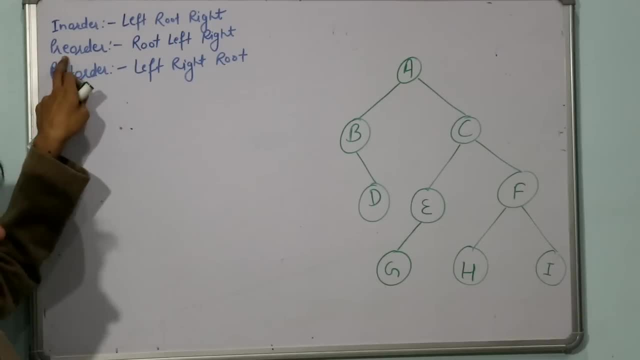 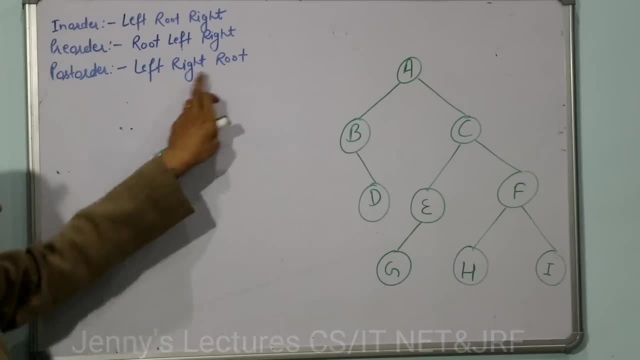 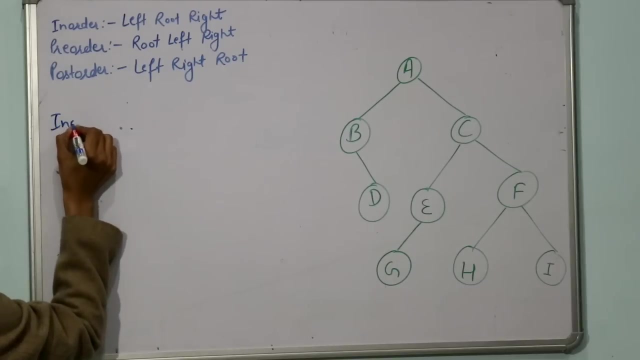 seen. in order: traversal of this single tree, this binary tree. Okay, And in order: traversal of this, this tree, this tree, in order: traversal of the tree. we would pass. So in order: traversal of the tree. in order: traversal of the tree first and then to and after: Okay, Okay, Okay, That's. 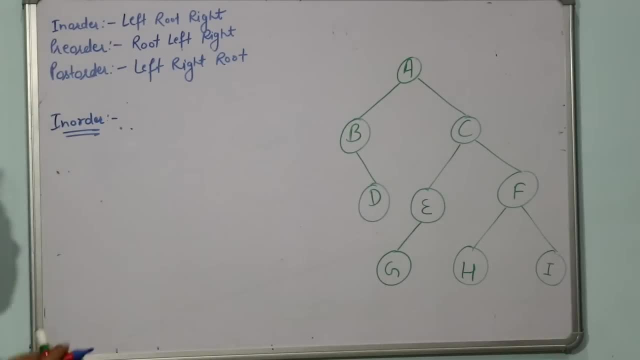 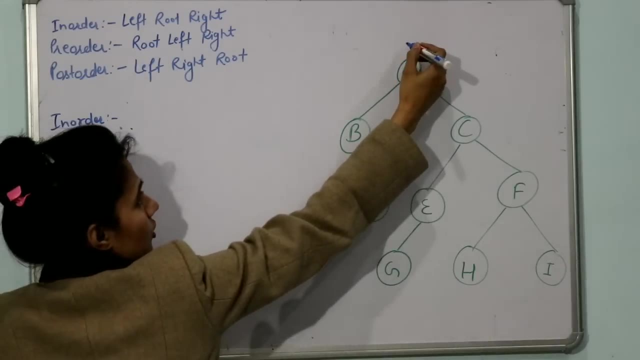 correct Pån the tree ofтам. lo mein beän tú Rate aur poani. demain is rồi lug受拉 here. you will start from a. ok in order. what will happen? first the left part will be reverse, then root, then right. so we will go from here. this is your root. you do not have to write root first. 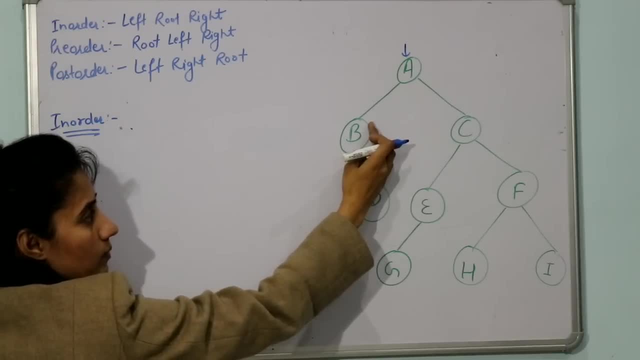 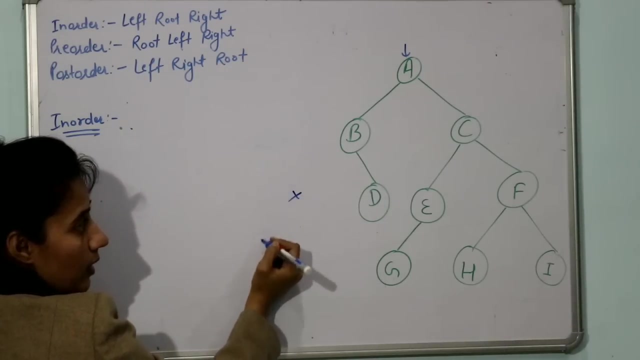 you have to traverse the left part so you will come to the left of it. ok, now, here you will check. obviously it is left, but here it is root for it. ok, we do not have to write root, we have to write left part. you will go to the left of it. there is nothing in the left part. it is null. left part. 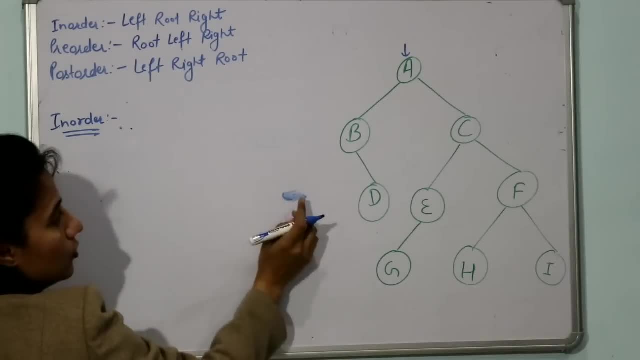 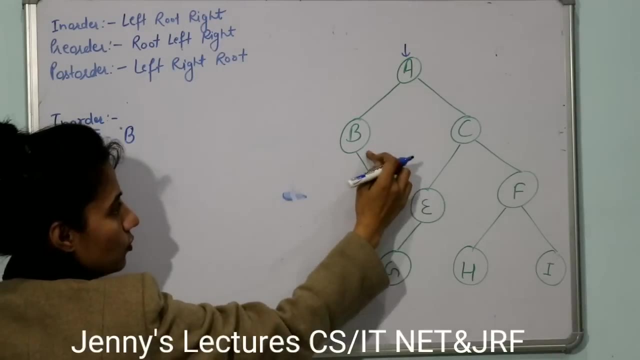 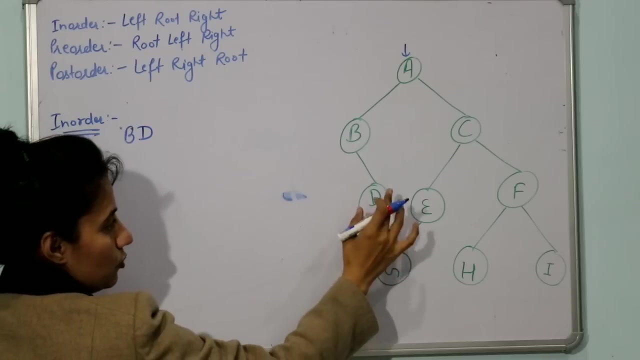 ok. so after that you would print root. root means you will print b. ok, what will you print after root? you will go to right part. what is in right d? ok, nothing in front. you will go back to b. you went back from b. you went to a- ok, 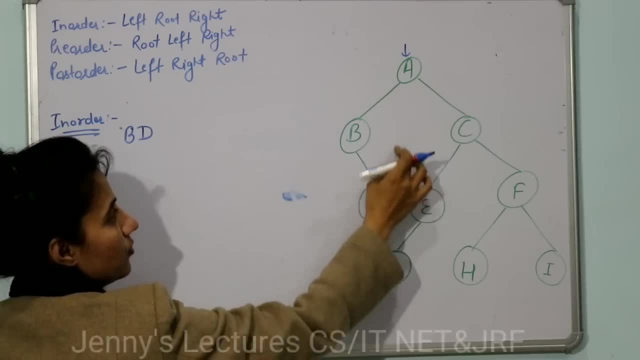 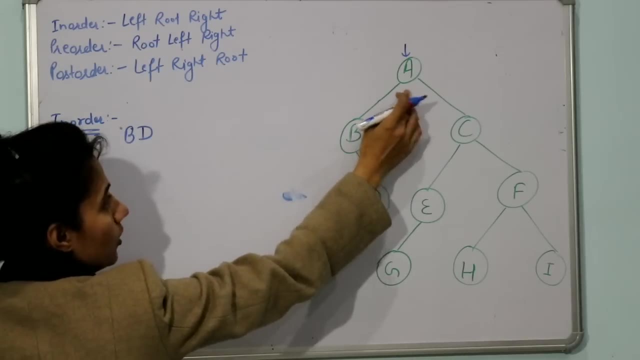 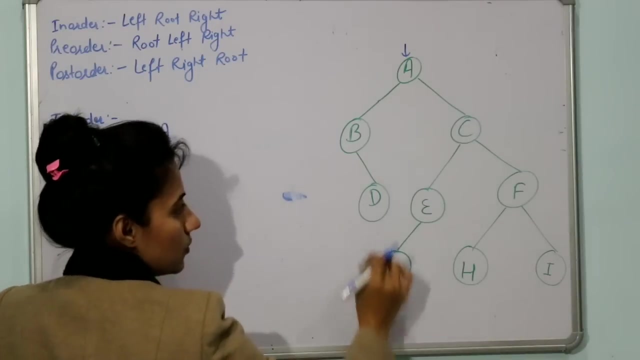 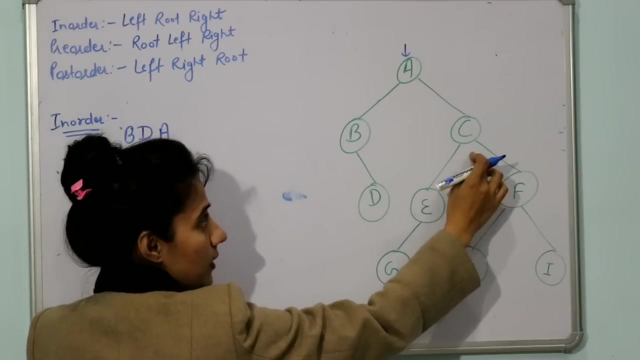 this is of a, that your left part is that of a. ok, now, if the left part is traversed, we will write root. root means you will write here: a ok, now you will go to the right part. this part, right, one right part, see, but for this right, this is right part, but this is subtree. 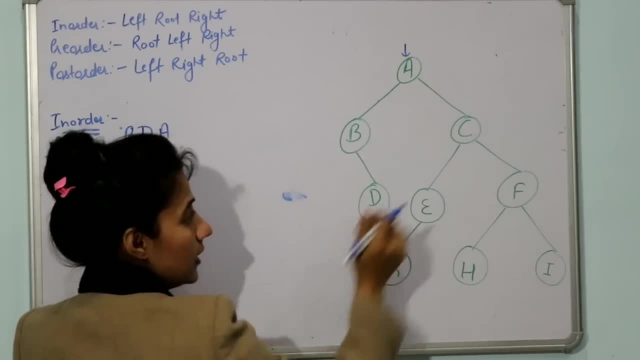 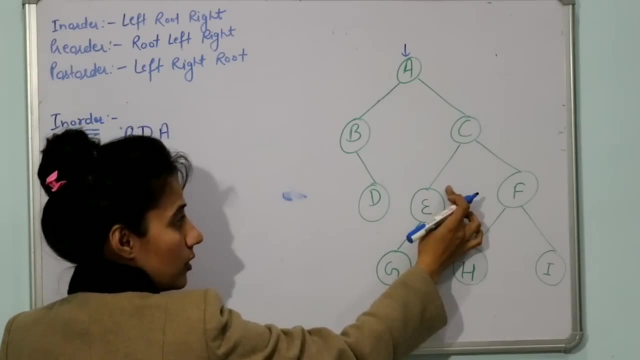 what is for the end of this is root, so you cannot write it directly. ok, Before this, what will come? Left will come. Now, this is the root for them, so you will go to the left of it. okay, Now, this is also the root for it, so you can't write it directly. Now, what will you go to in this? You will go to the left part. 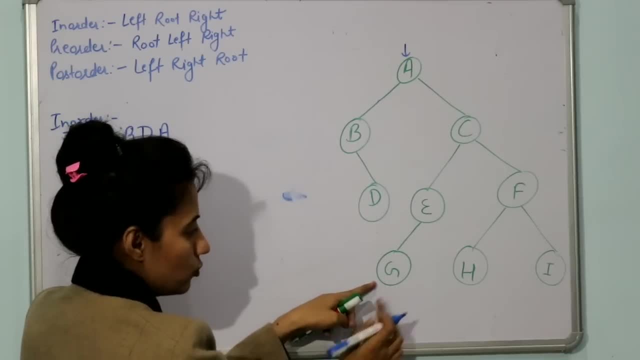 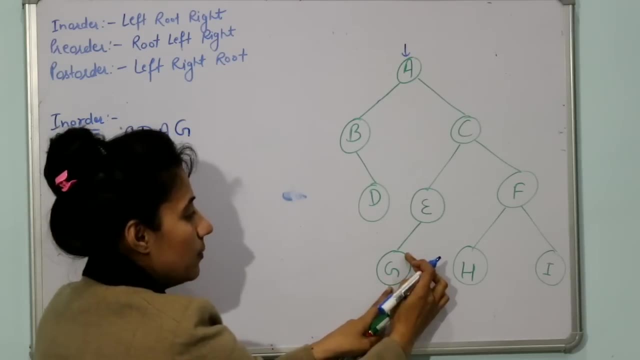 What is your G in the left After this? see, there is nothing in the left, so you will print G. okay, Left would be printed After the left. you will go to the back part and print the root Means. you will print E. after that, you will go to the right. There is nothing in the right, then you would print nothing. 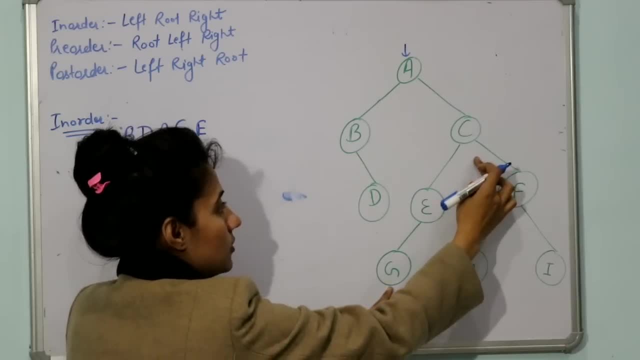 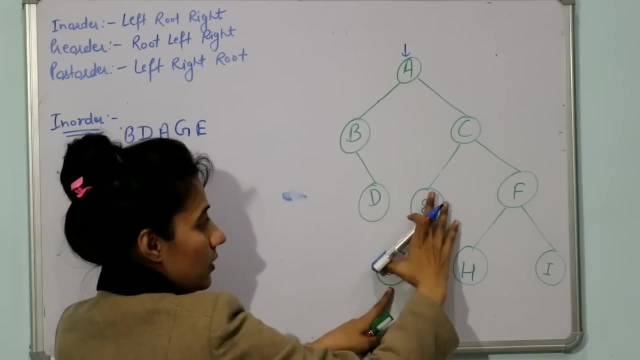 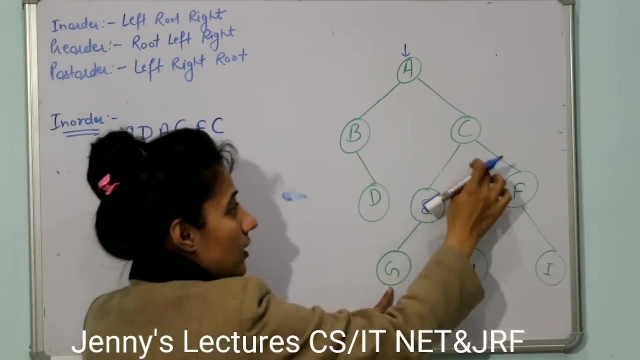 Okay, now back. you will go back from E here. See for this: root, what is this Left part? If your left is complete. after that, what would be printed? Root means C would be printed. After that, the right part would be printed. See for this. this one is the right part. 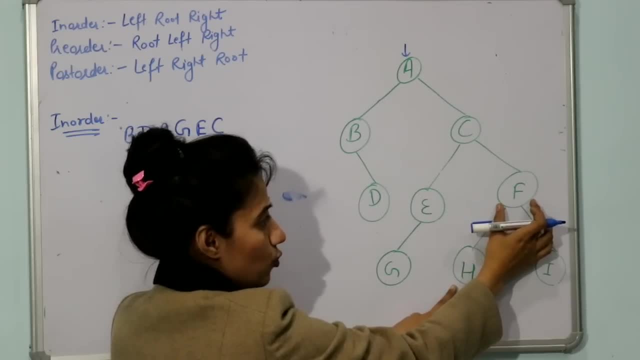 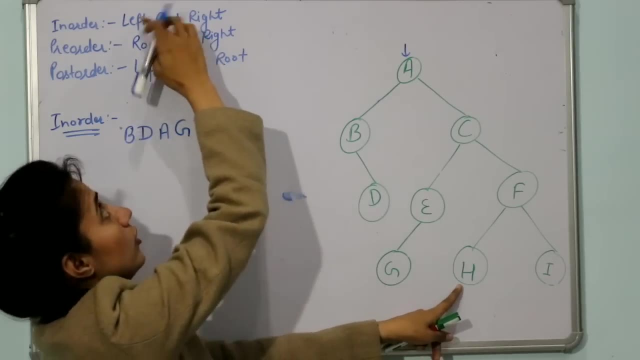 Right part. but you cannot directly print F, because F is the root here For H and I. there are two children of it, so this is its root. You will not directly print the root. before the root, the left is printed. 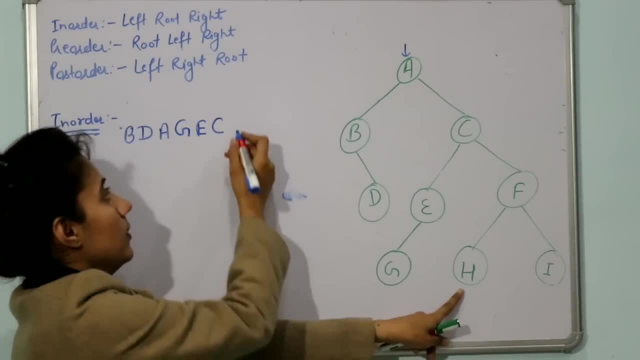 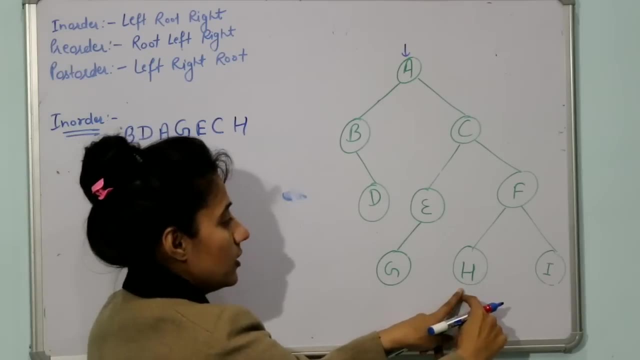 So you will go to the left of it, H. There is nothing in the left of H, so what will you print directly H. Then H is printed. after that, the left is printed. What is printed after the left Root? 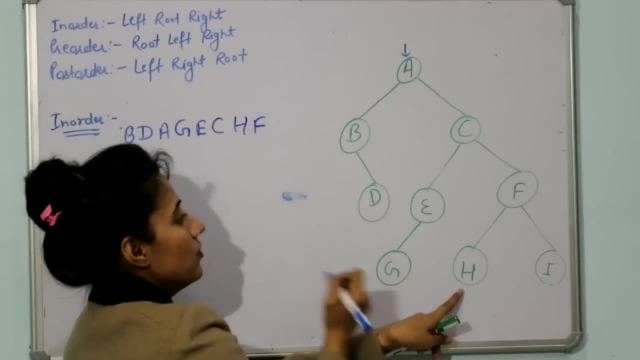 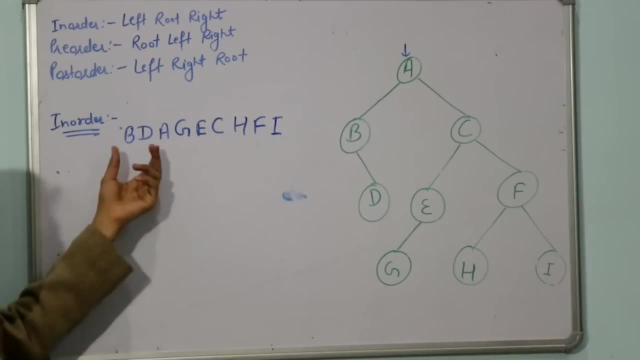 You will go to the back. your root is F. What will be printed after F? That is I Right one, So left root and I. This is the inorder traversal of this tree. Okay, Now what is pre-order? 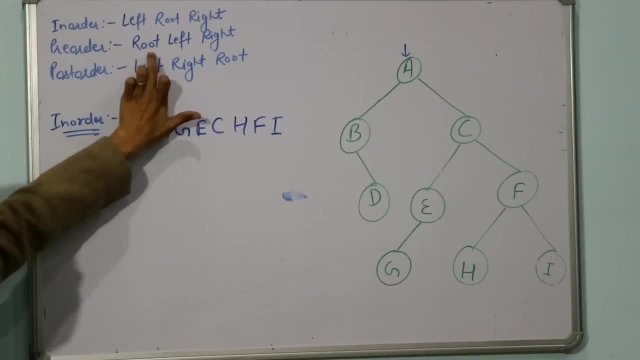 What will happen on pre? Pre means first. first root will be printed, after that left, after that right one. We will start from there, from the starting. Okay, Now root will be printed. So obviously this is our root. so what will we do? 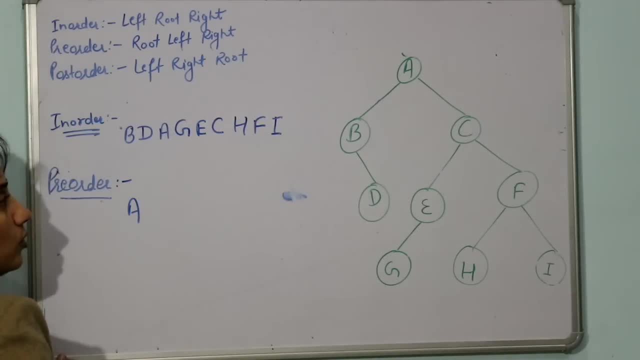 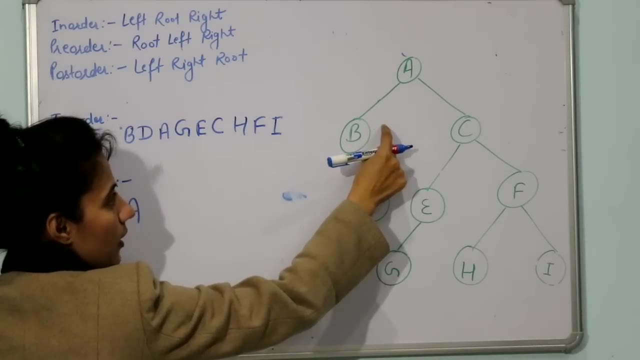 We will print A. What will be printed after root Left. Then you will go to the left part. Okay, Here you have come to the left, but what is this for? This is root, this is sub-tree, right? So for someone, what is this Root part? Okay, 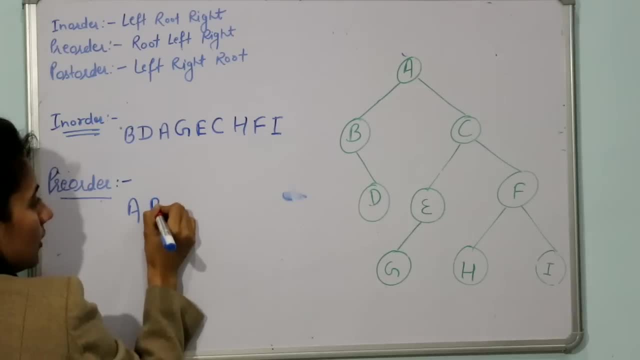 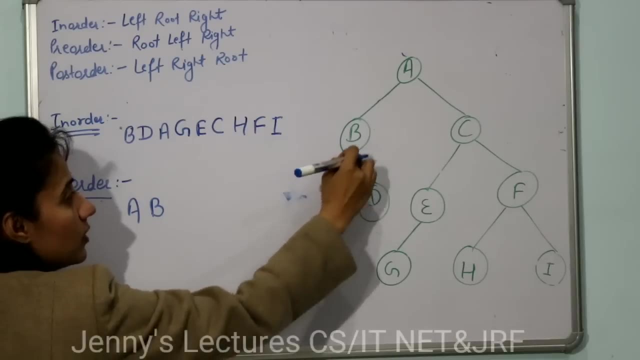 Still, we will print B, because root is printed first in this. Root will be printed after root: left. You will go to the left of this root. nothing is there, Null. Then what will be printed after? left, Right? 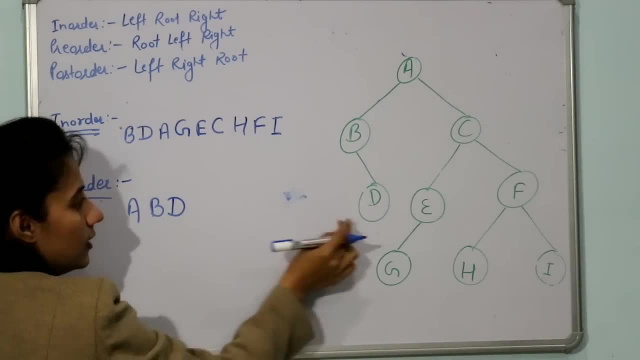 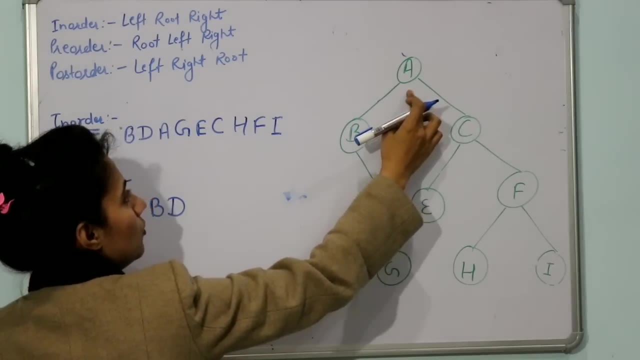 So you will go to the right of this. What is in the right, D, Then D would be printed After that. left right, nothing is there. Back to B: B has been printed. Back to A: A has been printed. 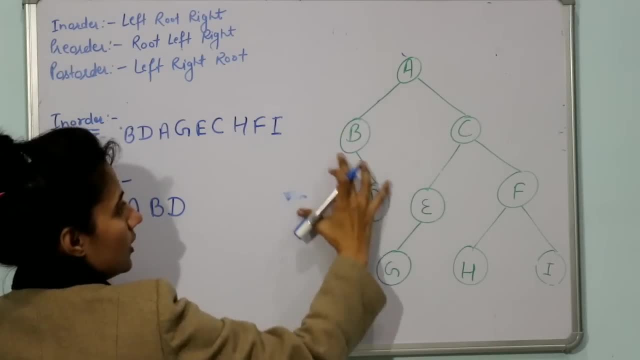 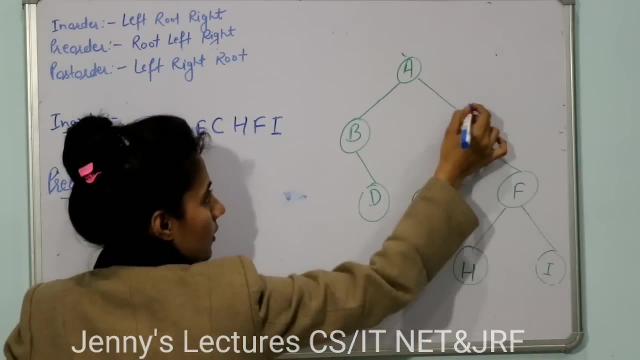 Root. this one was root. Root was there and for this left part was there. This was printed: Root left. After that, what will happen in pre Right part? This part would be printed. We will go to the right, Okay. 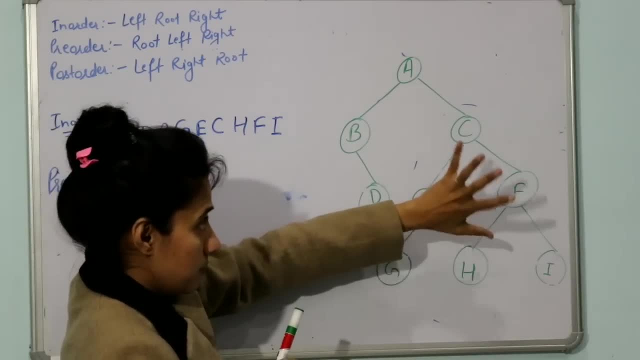 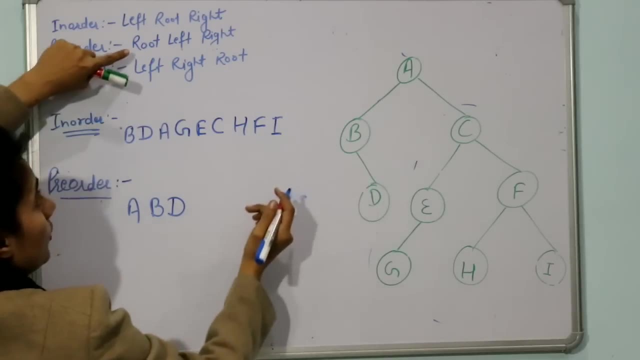 For this right part has been printed. Now C. What is this? C For E and F. what is this? This is root part. Okay, So in pre-order, root is printed first, Then C would be printed. 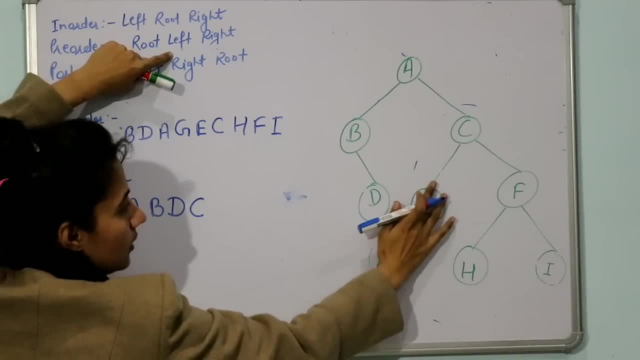 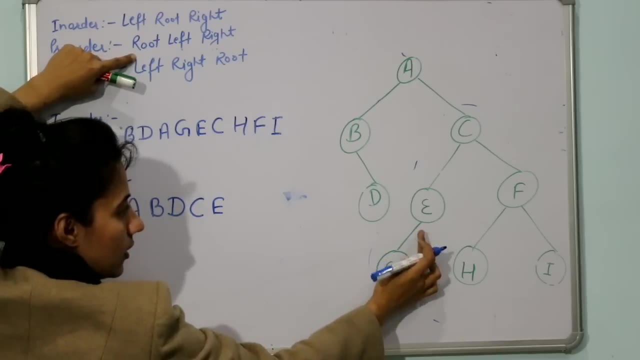 What will be printed after C Left? We went to the left. Okay, Left is this, But what is this For G root? So root would be printed E. Okay, Now, after root left, You will go to the left. 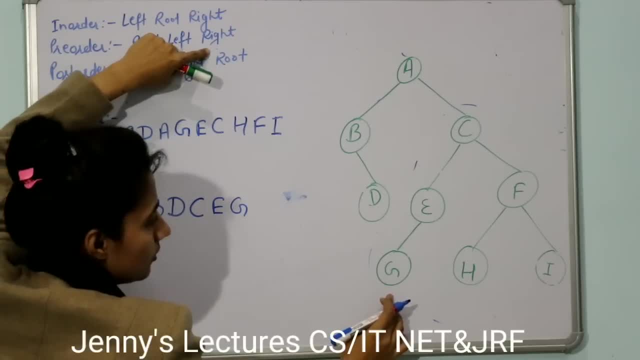 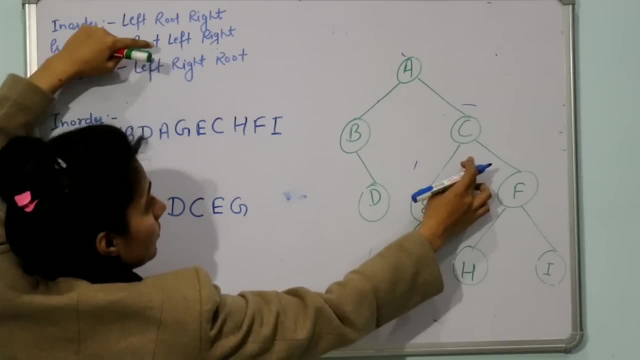 G would be printed. Nothing is there after this, After left in the right, So you went to the back track. Nothing is there in the right of E, So nothing would be printed. After that, back track again. Okay. 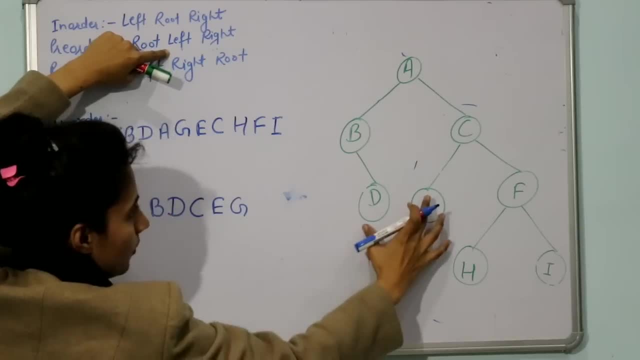 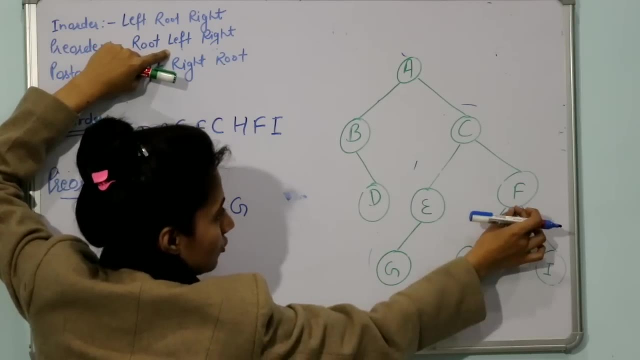 C. You have printed C Because root and left Root and this left part has been printed. After that, we will go to the right part. We went to the right part, But for H and I, this one is root. 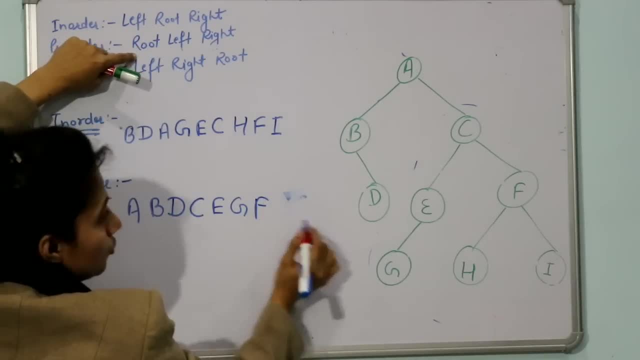 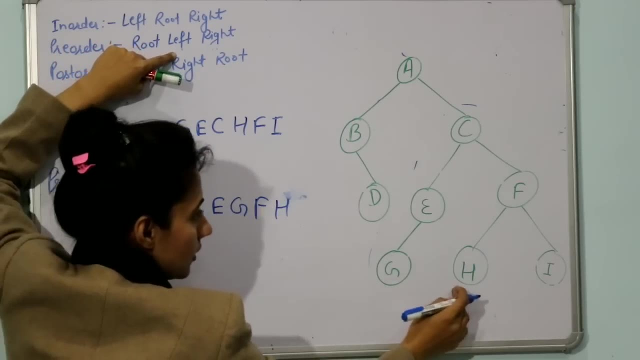 Okay, So what will be printed here? F- Root. We will consider this as root. Root would be printed After that left. Nothing is there in the left and right. Then H would be printed, Then root. 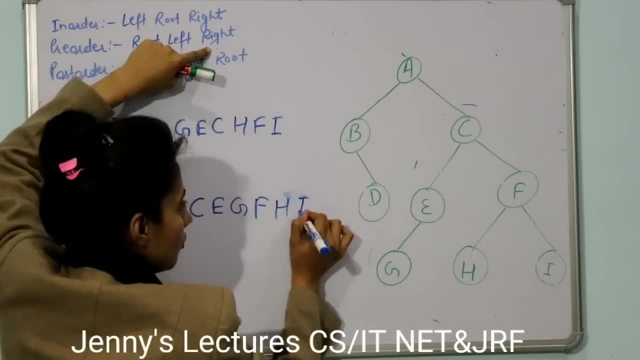 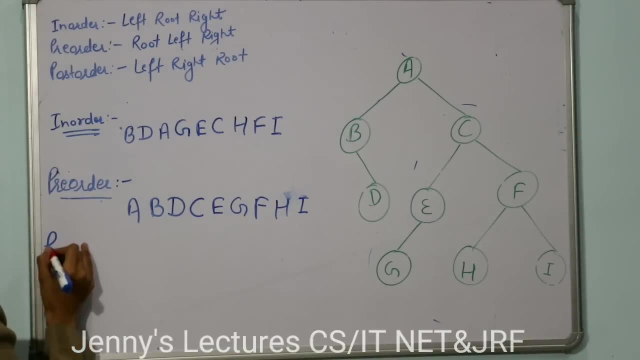 Left. After that this one is right part. Then I would be printed. So this one is pre-order of this binary tree Pre-order traversal. Now we would discuss this post-order traversal of this tree. Post-order means left, right. post happens later. 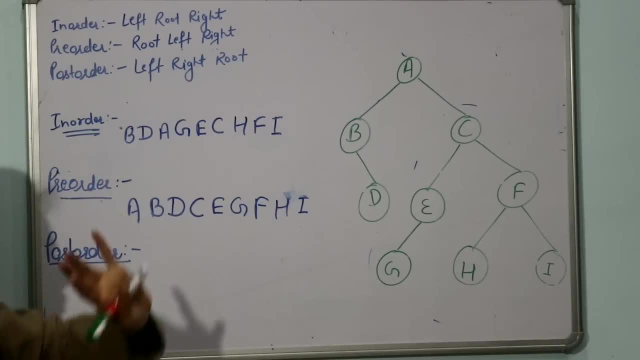 So root will come at the end. First left part, Then root part. You will start from here. You will not print the root Because it is at the end. You would go to left part. Okay, See, for this, it is left. 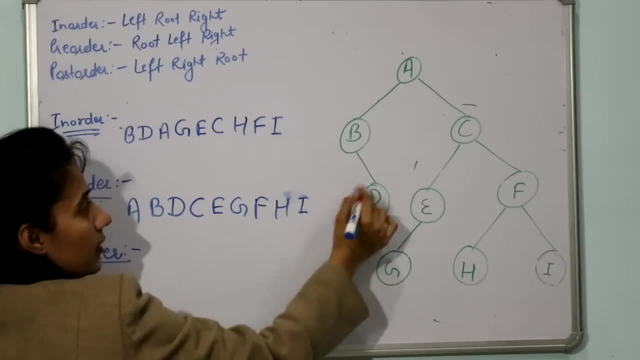 But this is also our sub-tree Because its children are D, So this is the root for D. Root will be printed at the end, So we cannot print B. Okay, First of all, left will be printed. 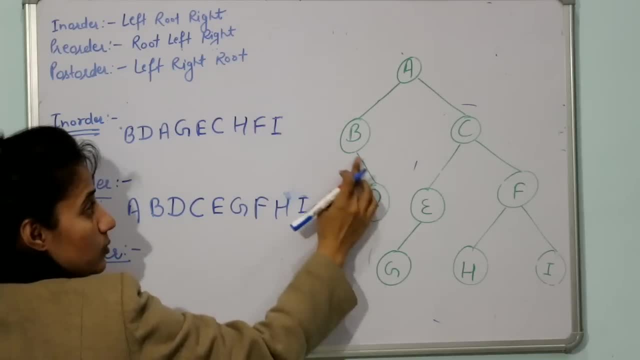 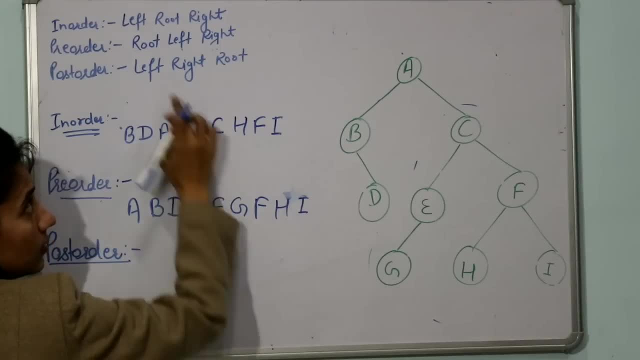 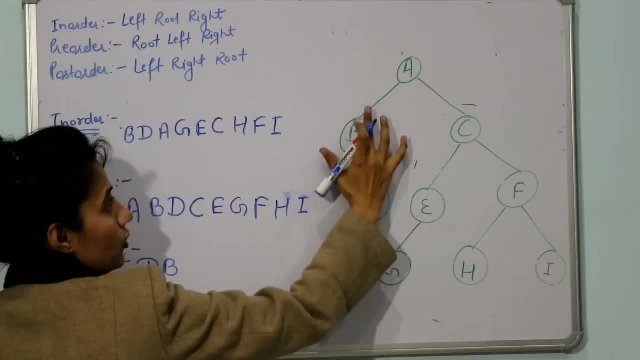 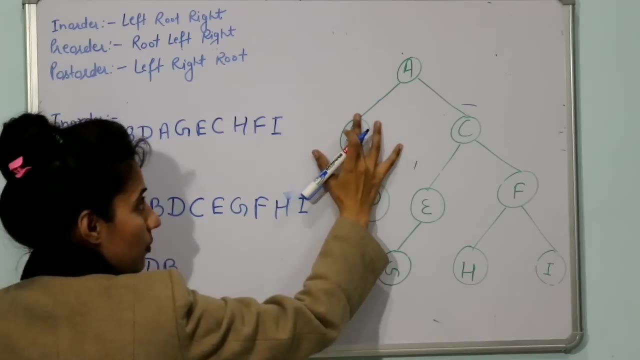 D is printed, Back part Means left part is printed for this root. Okay, Then right part will be printed for this root. Root will be printed at the end, So you will not print once Left part is printed. 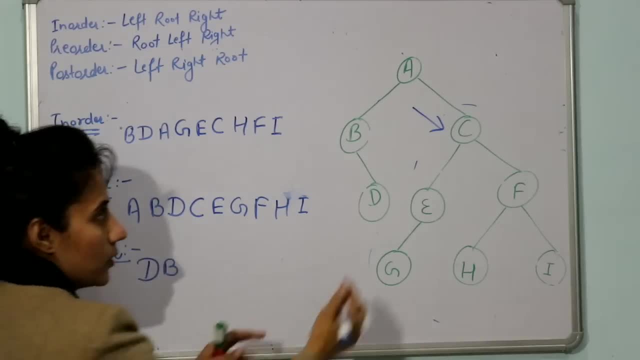 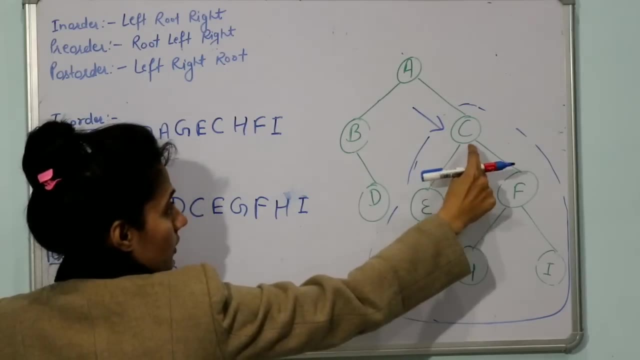 Then you would go to the left. This is the right part, This one, This one is the right part. Okay, Now C. See, Now there is C here, E and F. What is this? for all this? 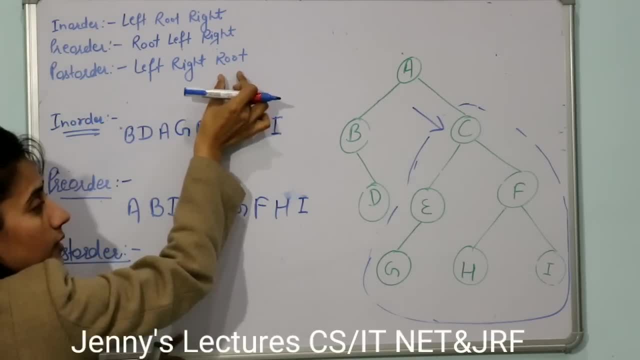 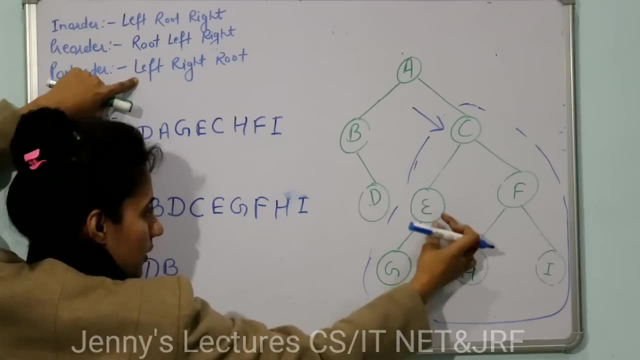 This is root, So we cannot print root, Because root would be printed in the last. What will be printed first? Left? Then you would go to the left part. You will go to the left side of C, But still this one is not left. 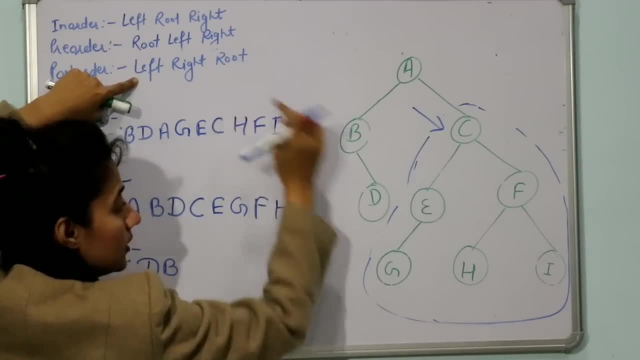 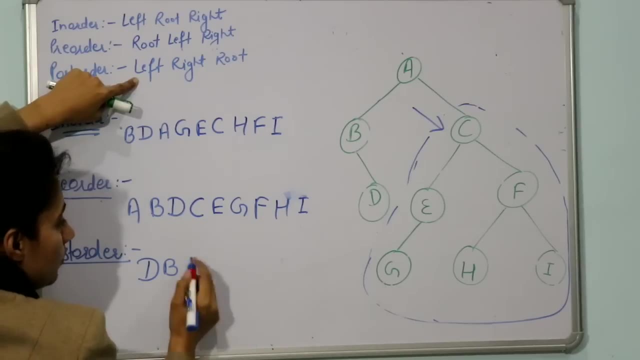 Because this is root for someone, This is root for G, So root would be printed in the last. So the last part is printed. The heart is printed again. you will go to its left. that is G. there is nothing in G left, then you print G left. 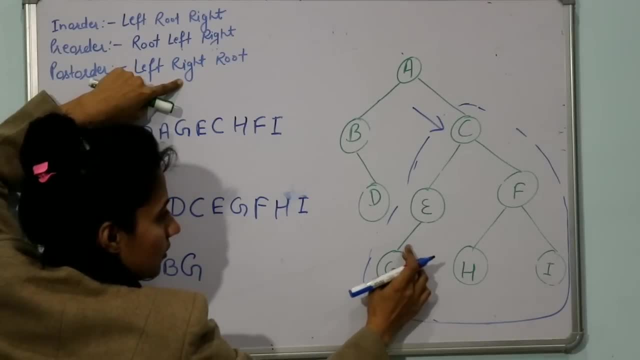 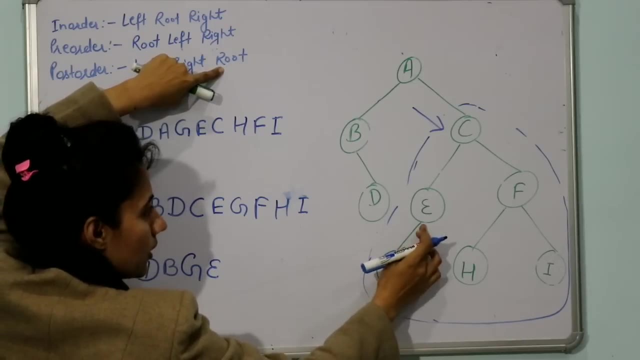 print is done. then right G print is done. left: there is nothing in the right of this root, so right will not print after that. what will be printed? root root means E is printed. ok, now G print is done. E print is done. now backtrack to C. now C root is: 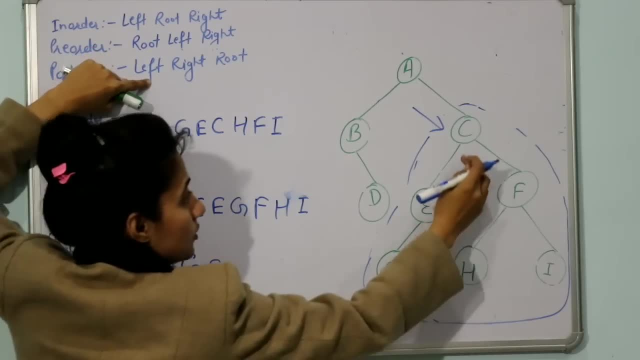 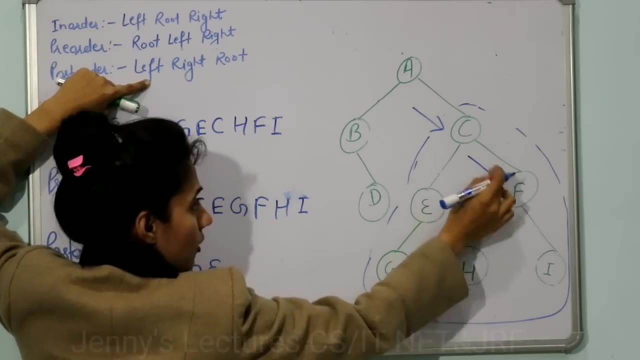 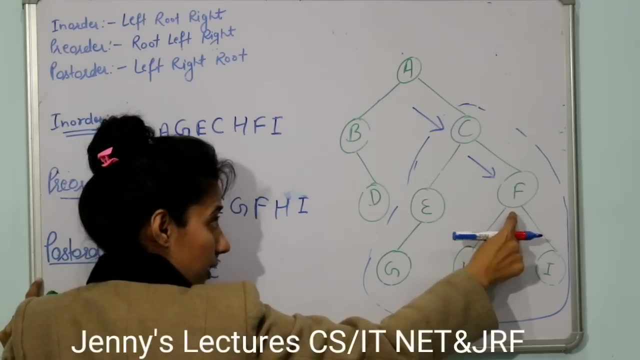 printed. C's left part is printed- left part. now C will not print because C is root. root will be printed at last after that, after left, you will go to the right part of C. ok, this one F H I right part, but this, what is yours, F is root for someone. what is for?